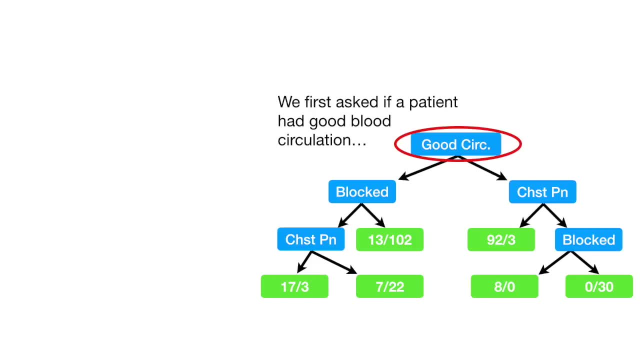 We first asked if a patient had good blood circulation. If so, we then asked if they had heart disease. If so, we then asked if they had blocked arteries, And if so, we then asked if they had chest pain. If so, there's a good chance that they have heart disease, since 17 people with similar answers did. 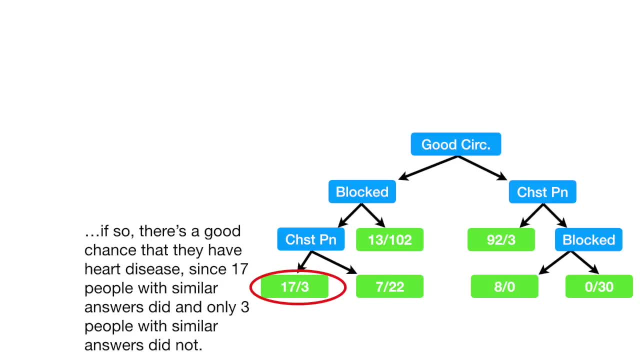 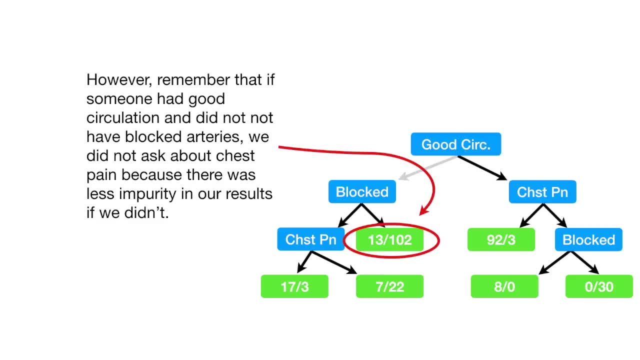 and only 3 people with similar answers did not. If they don't have chest pain, there's a good chance that they do not have heart disease. However, remember that if someone had good circulation and did not have blocked arteries, we did not ask about chest pain because there was less impurity in our results if we didn't. 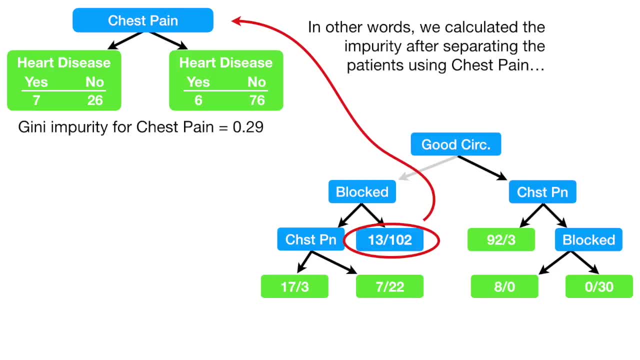 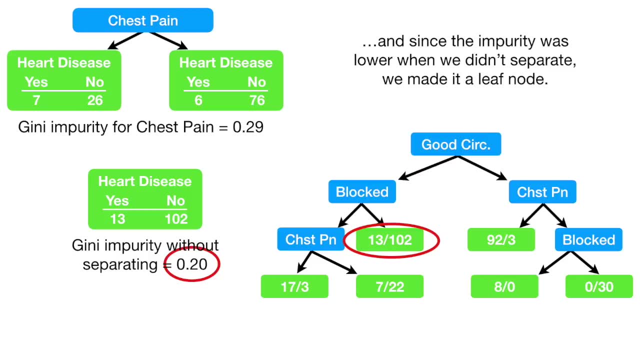 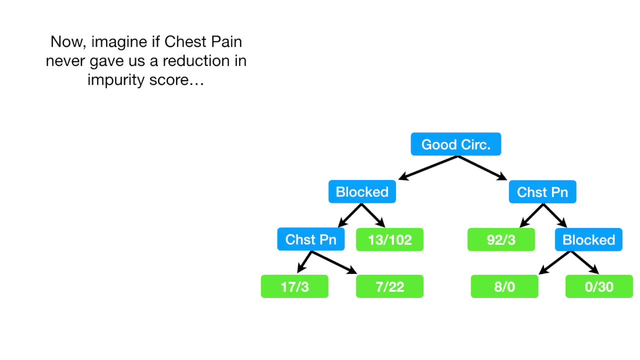 In other words, we calculated the impurity after separating the patients using chest pain. then we calculated impurity without separating And since the impurity was lower when we didn't separate, we made it a leaf node. Now imagine if chest pain never gave us a reduction in impurity score. 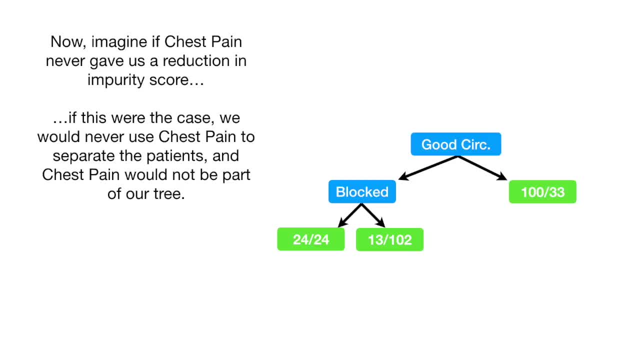 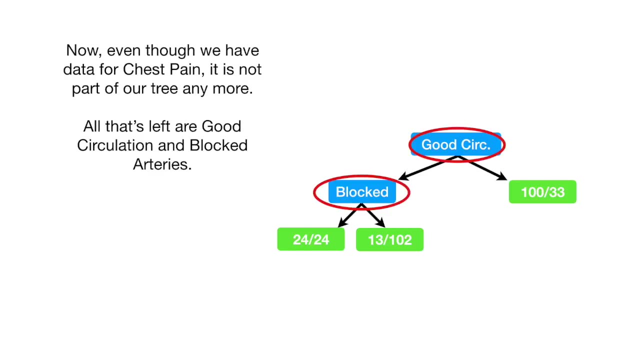 If this were the case, we would never use chest pain to separate the patients, and chest pain would not be part of our tree. Now, even though we have data for chest pain, it is not part of our tree anymore. All that's left are good circulation and blocked arteries. 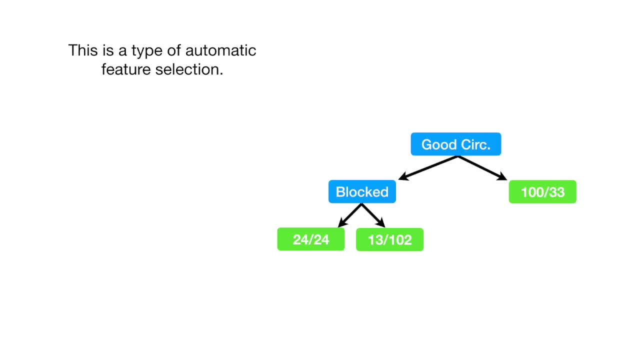 This is a type of automatic feature selection. However, we could also have created a threshold such that the impurity reduction has to be large enough to make a big difference. As a result, we end up with simpler trees that are not overfit. 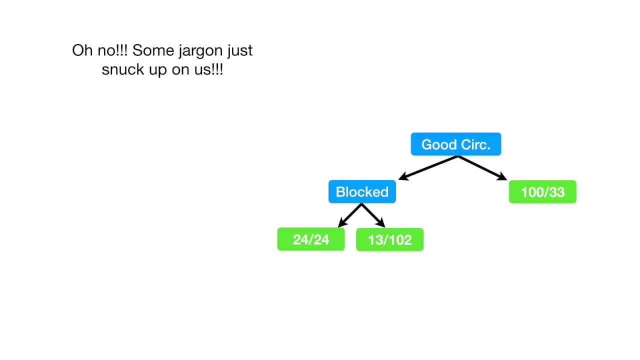 Oh no, Some jargon just snuck up on us. Overfit means our tree does well with the original data- the data we used to make the tree- but doesn't do well with any other data set. Decision trees have the downside of often being overfit. 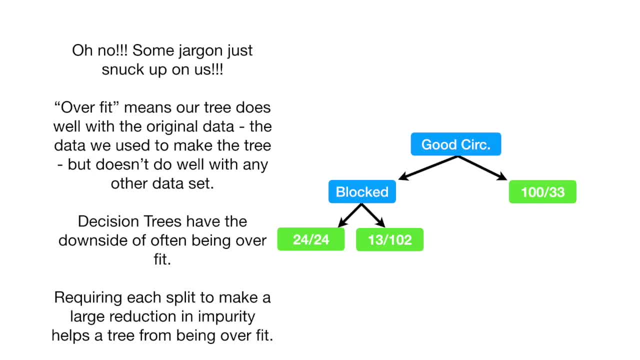 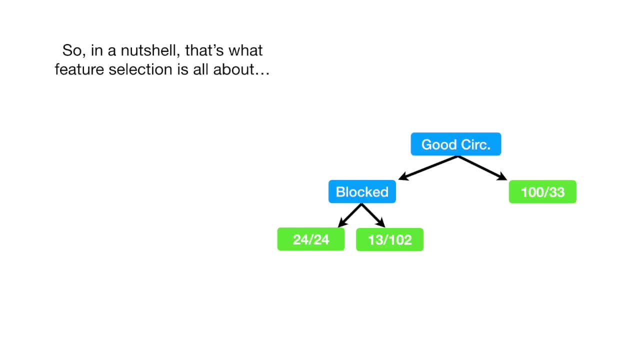 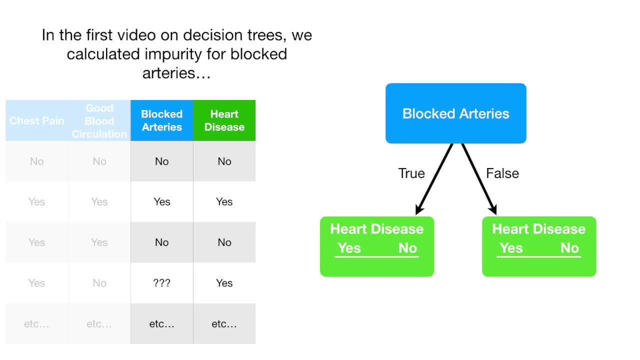 Requiring each split to make a large reduction in impurity helps a tree from being overfit. So, in a nutshell, that's what feature selection is all about. Now let's talk about missing data. In the first video on decision trees, we calculated impurity for blocked arteries.